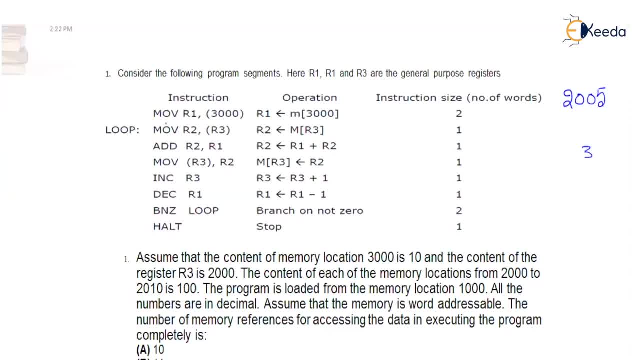 Let us have a look at this program. The first instruction is a move instruction which moves the contents of the memory location 3000 to R1.. The size of the instruction is 2.. Then there starts a loop. The loop will get started, So in the loop the first instruction is: 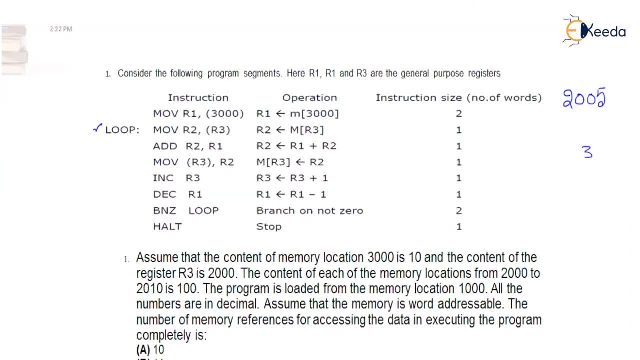 the contents of the memory of the memory location R3 will get transferred to R2 and the size of the instruction is 1.. Then R2 and R1 will get added and will get transferred to R2.. The size of the instruction is 1.. Move memory of R3, R2 does mean that the contents 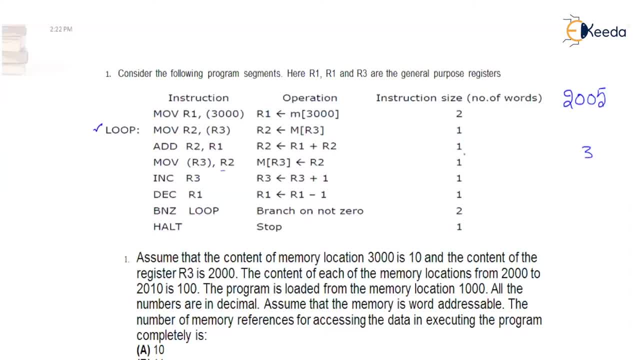 of the R2 will get transferred to memory of R3 and the size of the instruction is 1.. Next one is increment R3.. R3 contents will get incremented. R3 contents will get incremented, Which is instruction size is equal to 1.. And the next one is decrementing R1.. The contents: 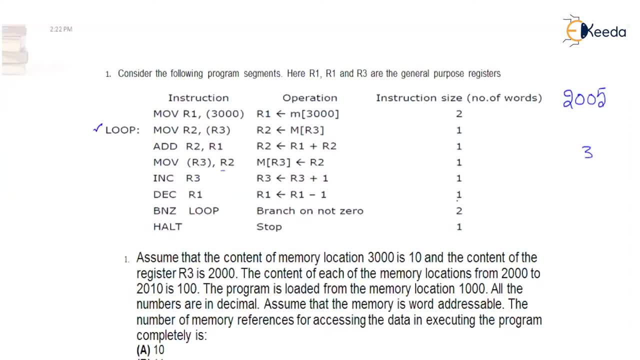 of the R1 will get decremented, in which the instruction size is one word And branch if loop, rather branch if non-zero. BNZ stands for branch if non-zero, Then we will go back to loop The label loop. So, branch or non-zero, we are going back to loop And the size of 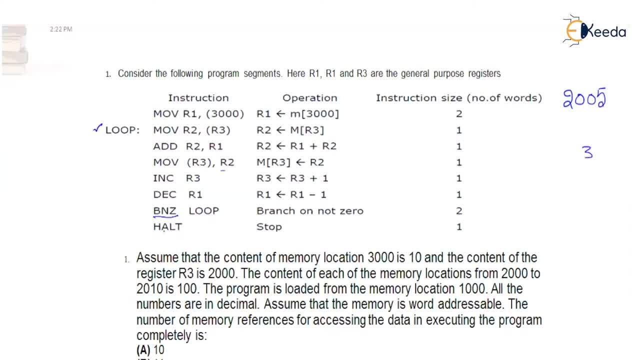 the instruction is 2 words And finally there is a halt. You know what is a halt instruction? Halt instruction is nothing but a machine halt which takes one word in the main memory. Now the first question is: let us have a look at, Assume that the content of the memory 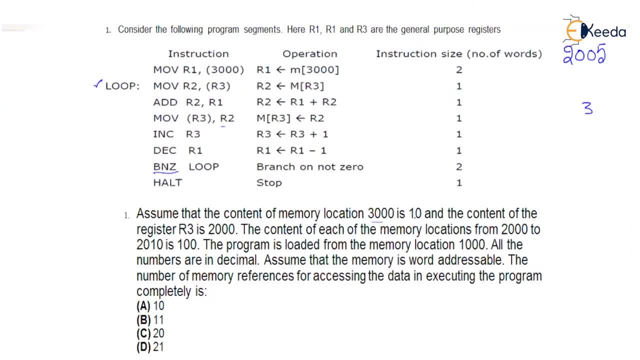 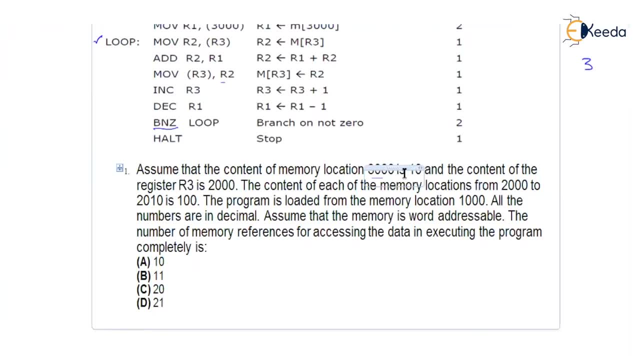 location 3000 is 10.. So here he has given the contents of the memory. location 3000 is 10.. He admitted that the contents of the memory location 3000 is 10.. Ok, And the contents of the register R3 is 2000.. Ok, Now I will put it here. I am going. 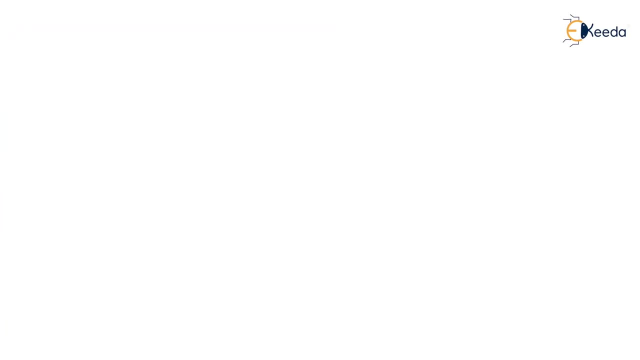 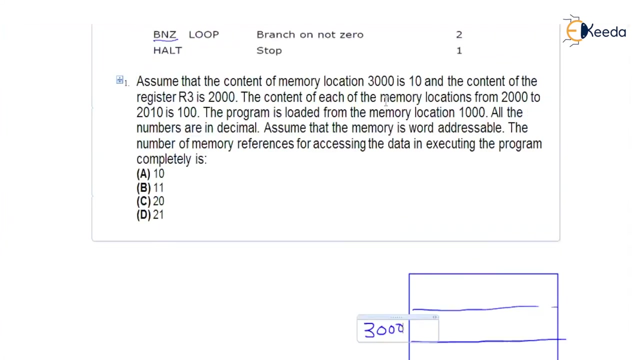 to use a memory block diagram. Let me draw the memory block diagram here. Here The contents of the memory location. Let me draw it. Let us say this is memory location 3000.. Let us see The contents of the memory location. 3000 is what? 10.. So the contents of the memory. 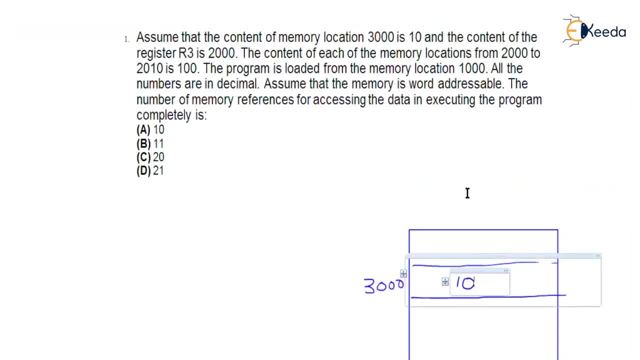 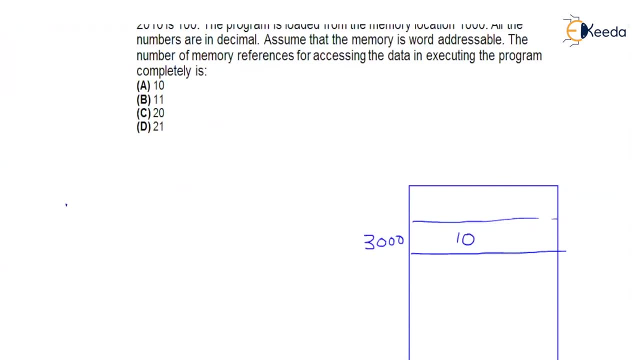 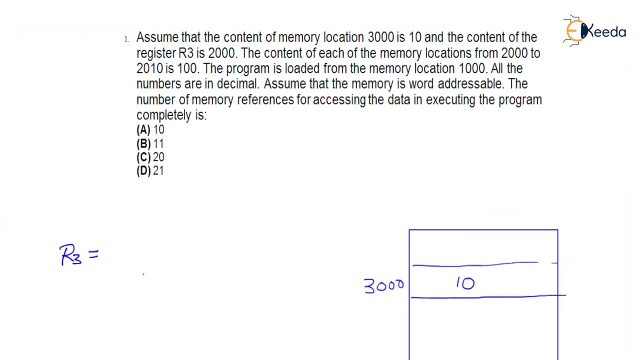 location 3000 is 10.. Ok, And the content of the register R3 is 2000.. The value of the register R3.. Let us take R3.. R3 is equal to 2000.. Ok, The content of each of the memory. 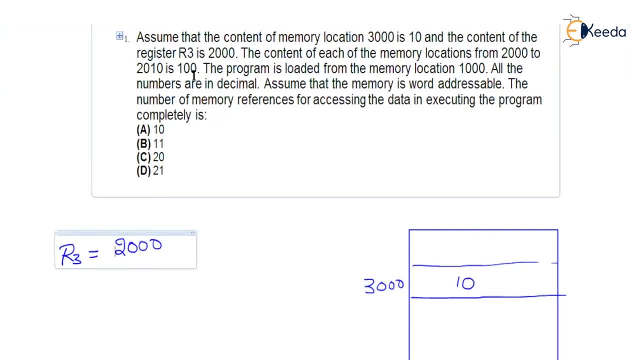 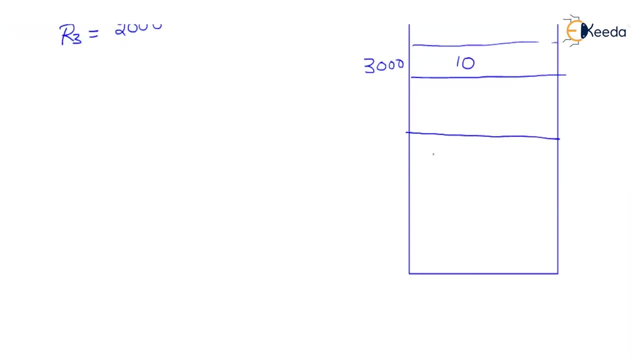 locations from 2000 to 2010 is 100.. So that is. there are memory locations. I am going to draw them. Ok, This is 2000.. Let us see. Ok, I did not chronologically order them. 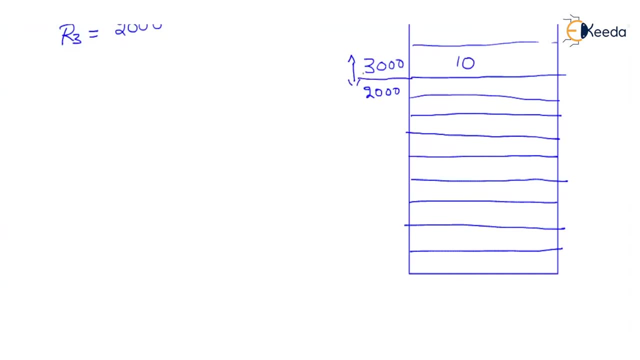 Of course. I mean this is a different memory, location 3000. And these are from 2000 to so on 2001,, 2002,, 2003,, 2004,, 2005,, 2006,, 2007,, 2008.. And I need to draw them, Ok, So 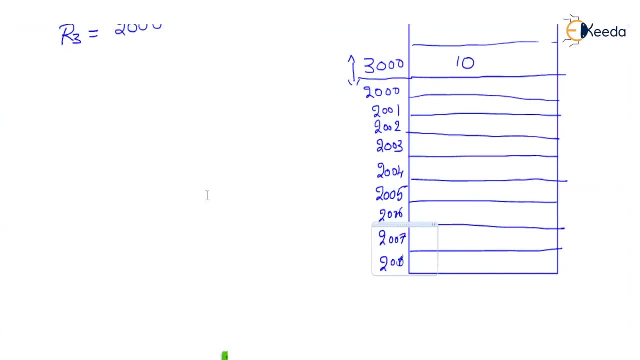 let me draw two more lines for making them 2000 to 2010.. Let me draw them. This is another memory location And this is followed by another memory location, That is, 2009 and 2010.. These are the memory locations. 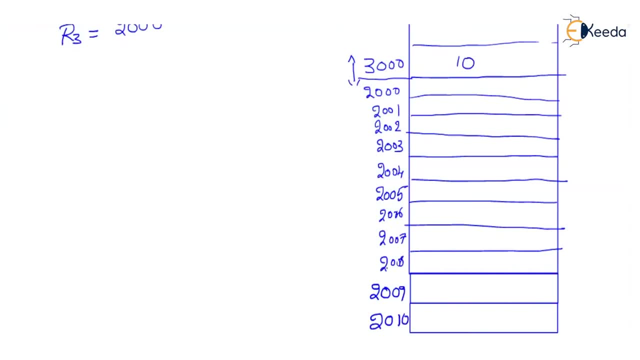 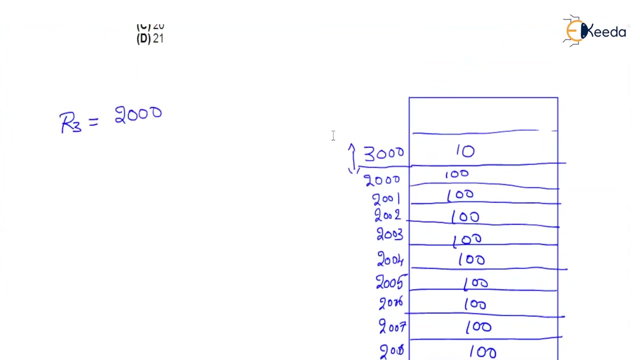 2001.. 2001 to 2010.. Each of the memory location content is 100, as it is given: 100, 100, 100, 100, so on. Yeah, This is the actual scenario of the system. Register R3 holds a value that. 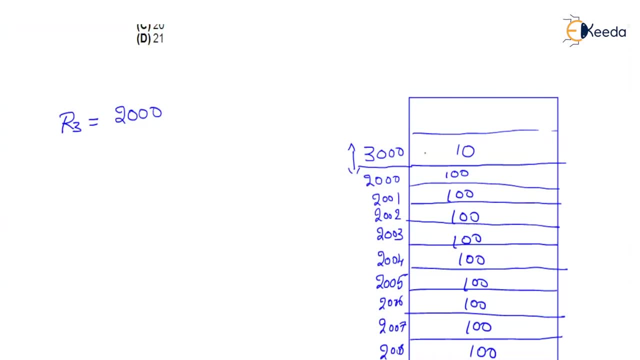 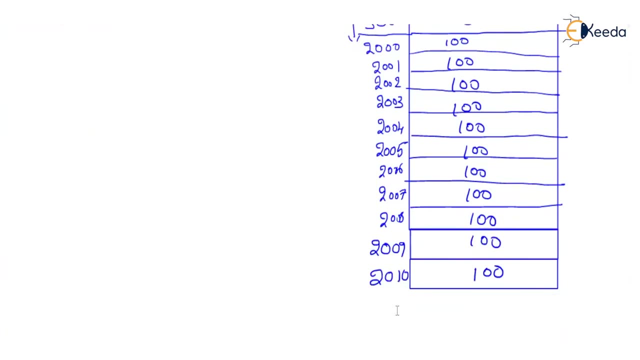 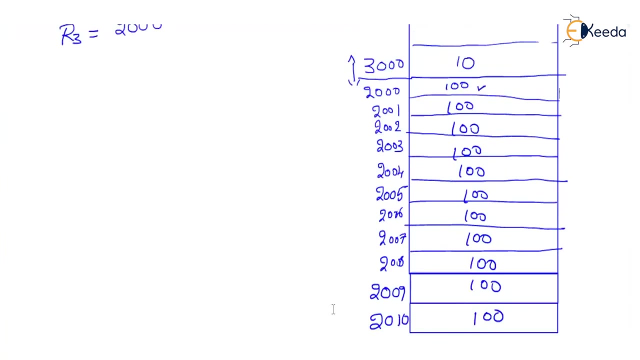 10.. When you go to the main memory, the memory location 3000 has a value 10.. And right from 2000 to 2010,, the every, each and every main memory location has the content, which is equal to 100 each. Ok, Now let us have a look at the question. now, The program is loaded from. 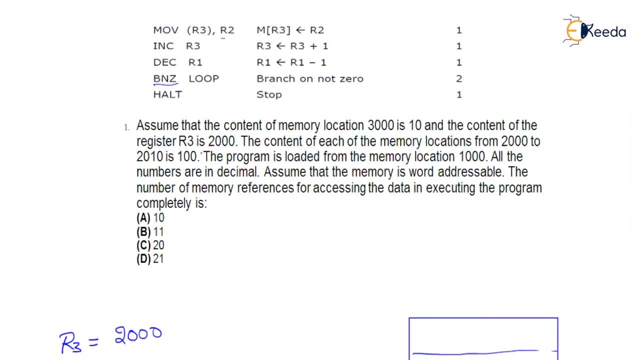 the memory location 1000.. Again, this program is also loaded from the memory location 1000.. All the numbers are in decimal. Assume that the memory location 1000 is a decimal. Assume that the memory is word addressable. it is word addressable. okay, the number of memory references. 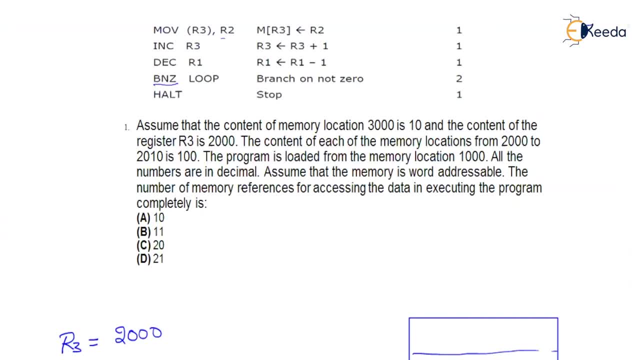 for accessing the data in executing the program completely? is this question? in the first question we are asked about the number of memory accesses, how many times we are going to access the memory for executing the program. we will just have a look at. so we will see when you execute this program. 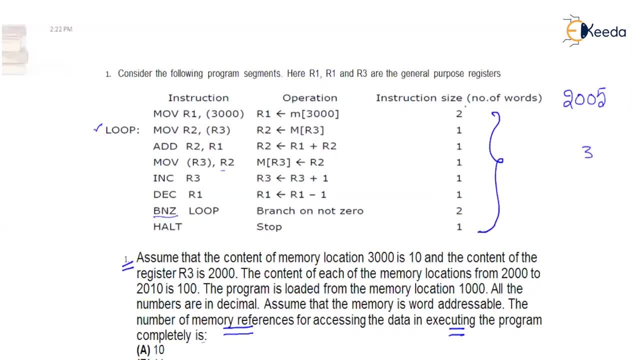 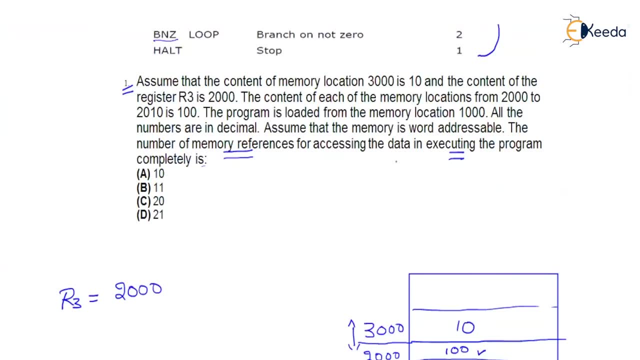 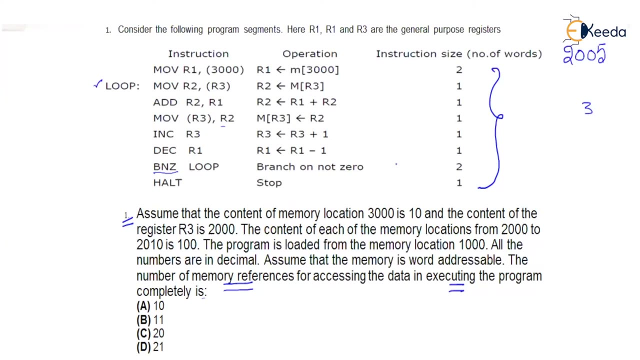 when you execute this program, all these instructions, how many times you are going to access the memory during the execution phase? this is the question. now, for that, we need to look at the memory accesses. we need to identify the memory accesses in the program. now let us start. 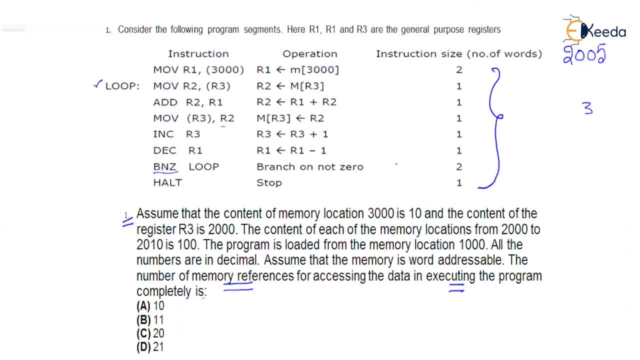 identifying collectively. you people also help me in identifying the memory locations. memory accesses: rather okay, the first instruction: does it have an access to the main memory? yes, it is main memory to r1, so this is a memory access. this first instruction will have a memory access, does it? does the second instruction have a memory? 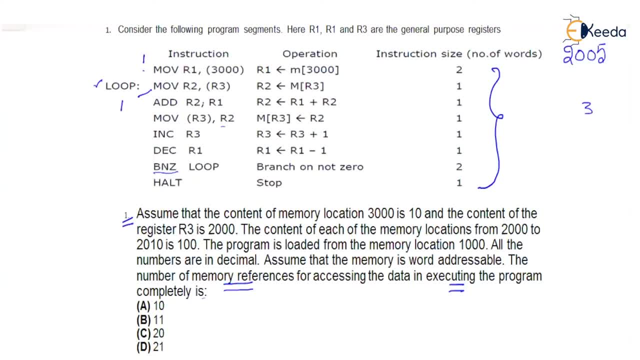 access. yes, this also has a memory access, because memory of r3 will get transferred to r2, and does this have a memory access? no, this instruction doesn't have a memory access. okay, because simply the contents of the registers are getting manipulated. that's it. there is no memory access, you can see in executing this instruction, but here there is a. 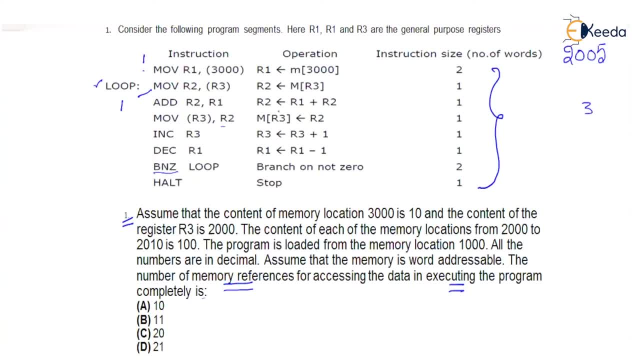 memory access, that is, r2 will get transferred to m of r3. so again there is a memory access right now you can clearly see. of course the rest of the instruction doesn't have any memory access because r3 contents are getting manipulated simply. simply incrementing r1 contents are 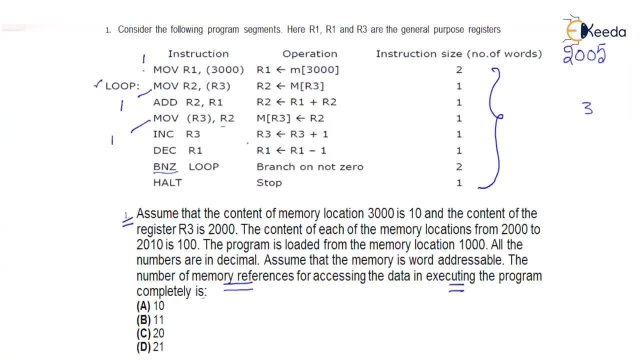 simply getting decremented and manipulated. so here in these two instructions are the followed. these two instructions doesn't have any memory references whatsoever. okay, now let us have a look at this total number of memory access. this is one. this is one. this is one. okay, total number. 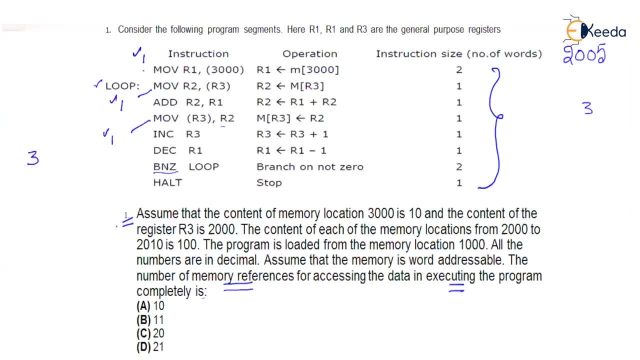 of memory access are three. okay, but if you can have a clear look at this question, let me show you something. these two memory accesses are within the loop- okay, and these one access is outside the loop- okay. now, when executing the program, if you want to know all together there will be how many memory access. you need to understand how many times this loop. 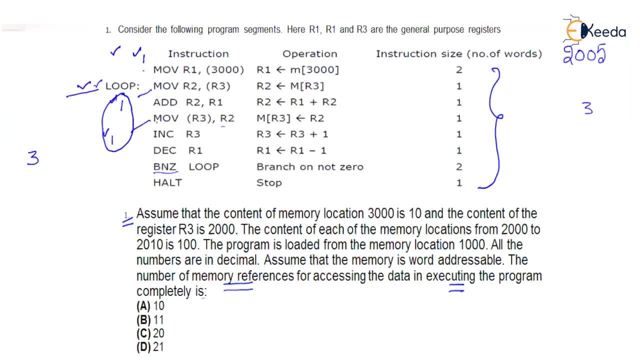 gets repeated. okay, just look at the program. when you look at the program, loop will get repeated on the value of r1. okay, after decrementing the r1, if the value is not a zero, then we are going to loop. if the r1 value is zero, then the loop gets terminated again. this loop depends on the 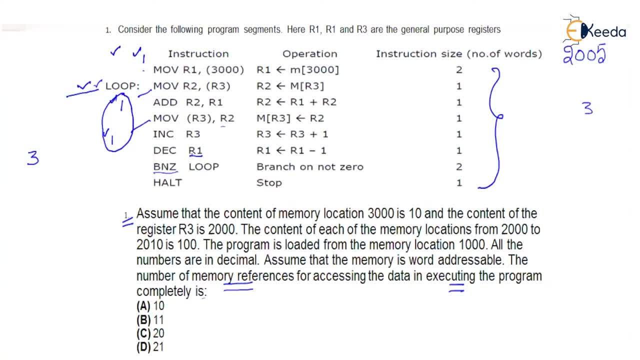 value of the r1. every time r1 gets decremented then we are going to check with the condition. if the r1 is equal to zero, then we are going to terminate. if the r1 is a non-zero, this is non-zero- then we are going to go back to the loop. so loop is going to get repeated for r1 times. 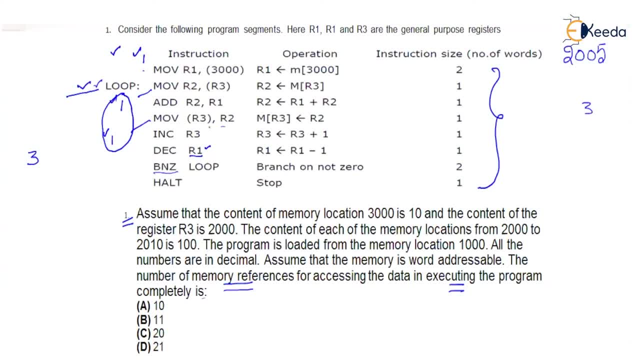 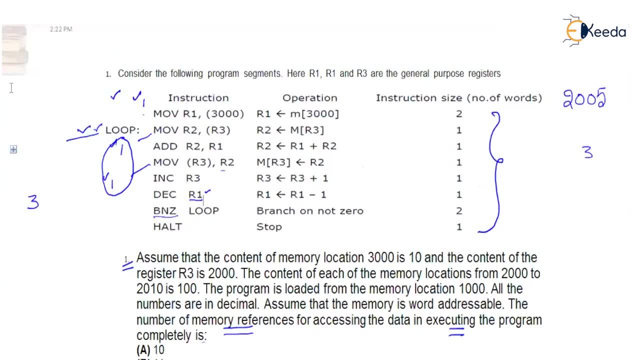 okay, the moment r1 reaches to zero, loop gets terminated. okay, so we will see what is the value of r1. okay, if you can have a look at this program, the first instruction itself transferring the contents of the memory location 3000 to r1. right, so the r1 value is equal to memory of. 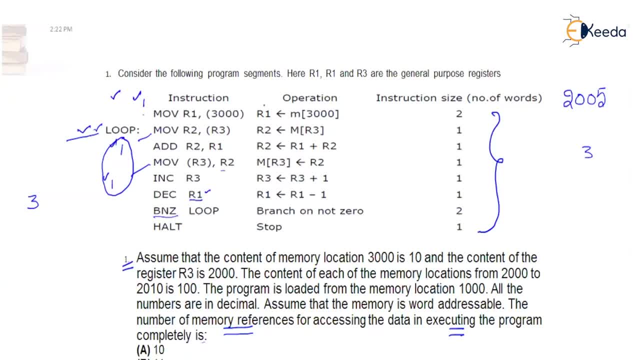 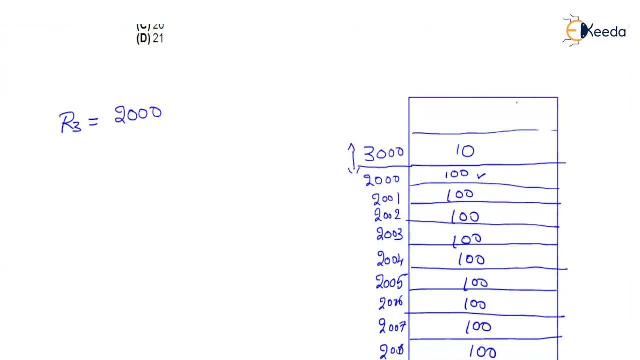 3000 right. memory of 3000 is getting transferred to r1, which is the first instruction, so r1 will be initialized by the value of memory of 3000 right, so which means that memory of 3000, which is equal to 10, will get transferred to r1 during the execution of the first instruction. 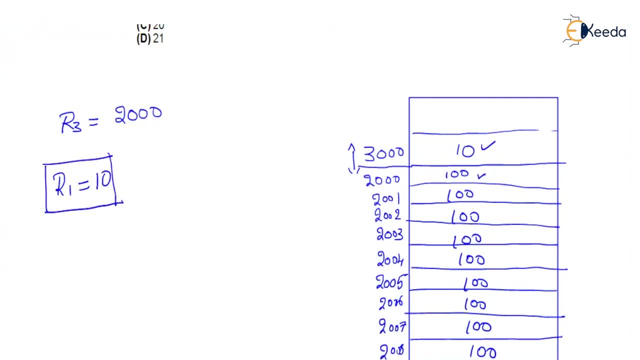 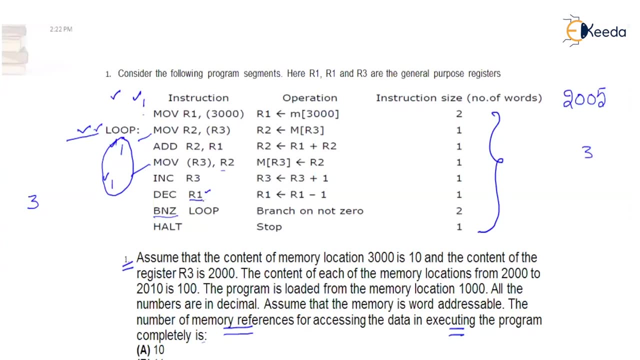 so r1 value is equal to 10. so every time when one of the iteration of the loop gets transferred to r1, then the value of r1 is equal to 10. so every time loop is getting finished, r1 is getting decremented. so finally, loop is going to repeat it for 10 times. 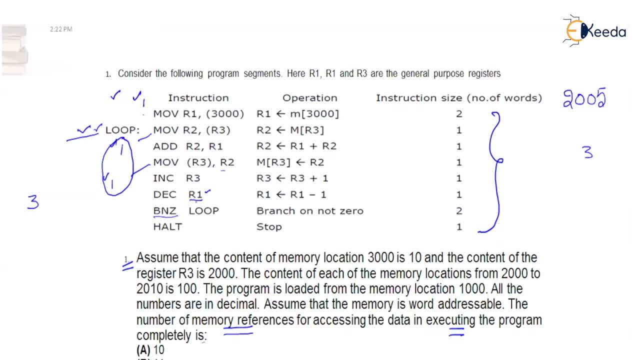 and after 10 times, r1 becomes zero. the moment r1 becomes zero, loop gets terminated. so that means that loop is going to get repeated for 10 times. okay, during which in the loop, inside the loop, there are two memory access, right? so total number of memory access will be: 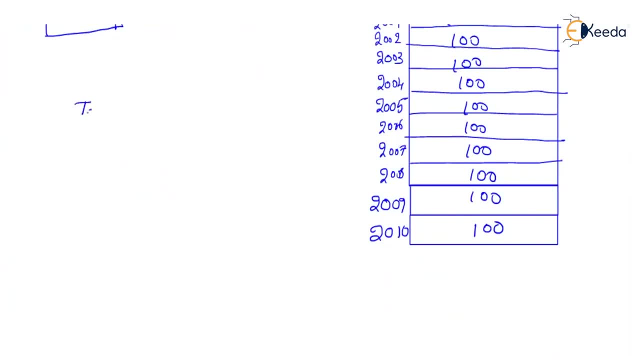 I will write it here, is equal to 2 into 10 plus 1, that is two. memory access are within the loop. loop is going to get repeated for 10 times. so 2 into 10 plus 1, that is equal to 21 clock cycles. r1 is going. 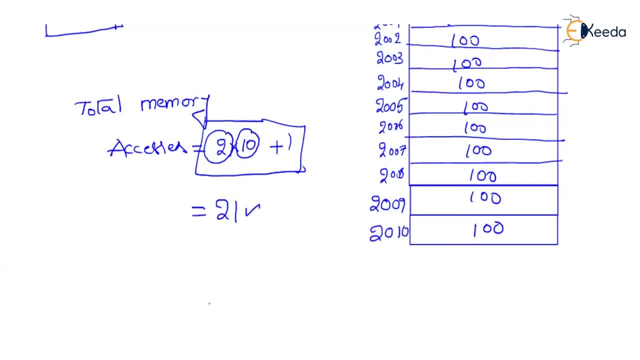 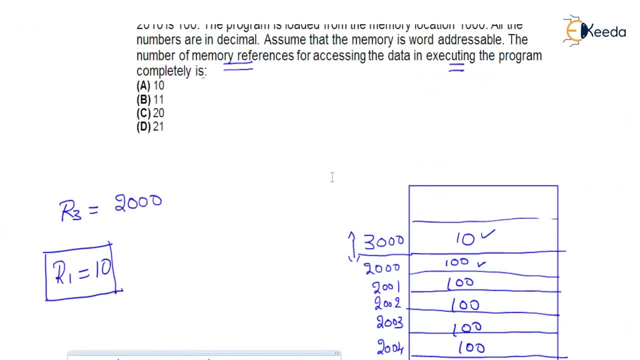 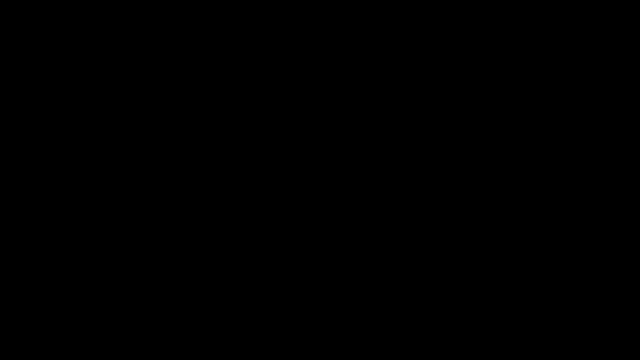 to get repeated for 10 times. sorry, 21 memory access- rather okay. so in this program the memory is going to be referenced for 21 times during the execution. this is it. so r1 and r1 are here. so r1 and r1 have been remembered in this program and r1 have this. one was here and r1 is going to get repeated for 21 times, so r1 is going to get read this one, but the next one has to be read after r1 as well. the next one has to be read like r1 and r2 after r1, so r1 is going to get read after r1 and r2 and then r1 has to get read. after r1. so you can see from the default the same way. but for now they are all read together so they are not nearly exactly same as the original. so they are all read in the same just the same. so, for example, r1 have been read in the normal order and then r1 is going.